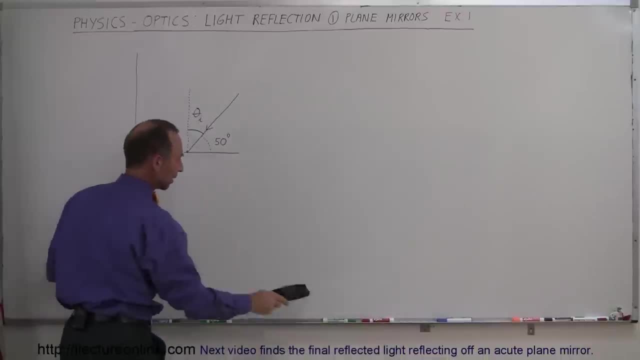 and let me make sure I make it the same. I wasn't going quite in the right direction here, so let's make it look like this. that's much better right there. so this was the angle of reflection, theta, sub r for reflection, And we know that those two have to be equal to each other. well, if this is 50 degrees, then this: 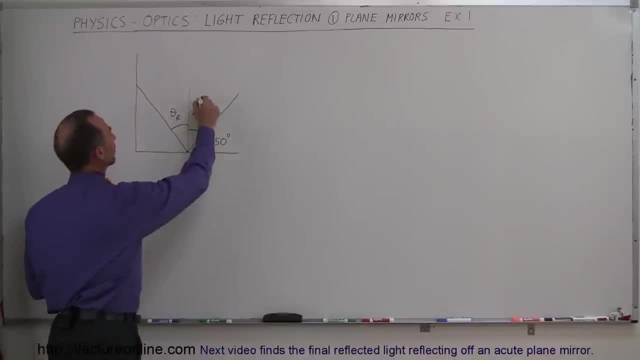 angle has to be 40 degrees. 90 minus 50. that makes this a 40 degree angle, which means that this also must be a 40 degree angle. so what is the angle of incidence against this mirror? right here again, we draw a perpendicular to the mirror and we're trying to find out what this angle is equal to. 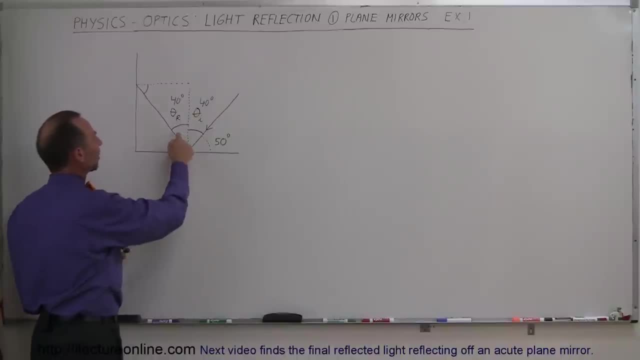 angle of incidence. the best way to do that is to go ahead and say: well, what is this angle right here? a 90 degree angle, 90 minus 40 makes this a 50 degree angle. we know that this is the right angle, or 90 degrees, and we know that the sums of the angles of the triangle add up to 180, which means 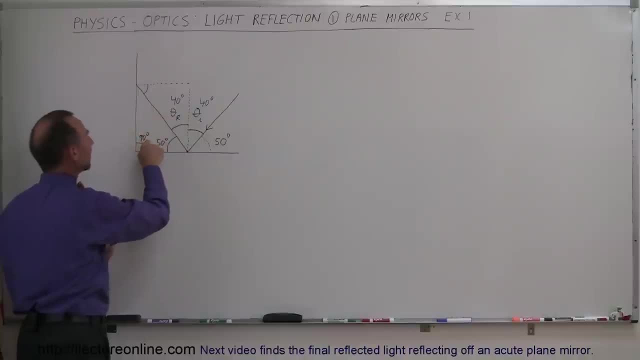 that this angle here has to be 180 minus 90 minus 50, so 180 minus 90 minus 50 degrees, which is 40 degrees, which makes this angle a 40 degree angle, which makes this angle, therefore, a 50 degree angle degree angle, because the two add up to 90, so this is a 50 degree angle, which means that the 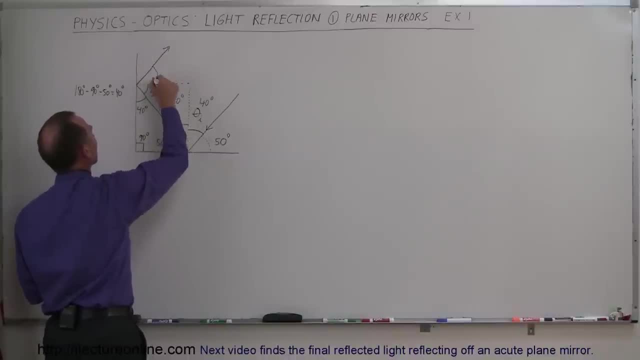 reflected beam right here will have an angle of reflection over here of 50 degrees, which means that the exiting angle has an angle of 50 degrees above the horizontal, and that's how we follow those. the light rays through a corner reflector, as we call it. that's kind of a typical corner. 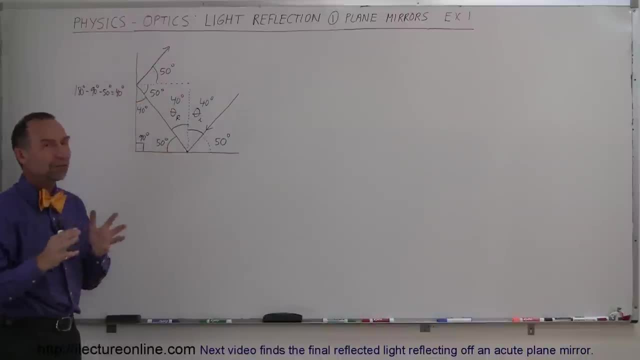 reflector where ray comes in and reflects off and then goes back roughly the same direction that it came in on. now we can see how we go ahead and do that in a very simplistic situation. now what we do if the second mirror is not directly upward or perpendicular to the first mirror. what if 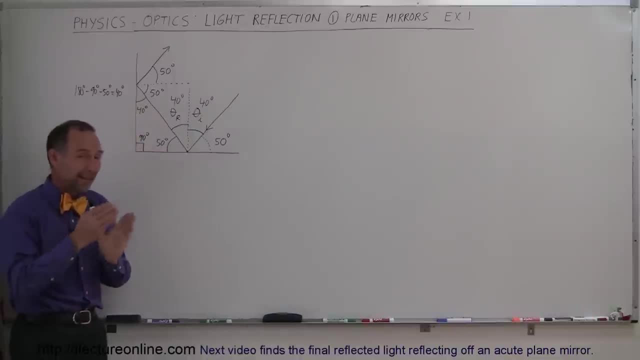 it's angled inward or angled outward. well then, we have to take care of that differential in the angle, and on the next videos I will show you how to do that. 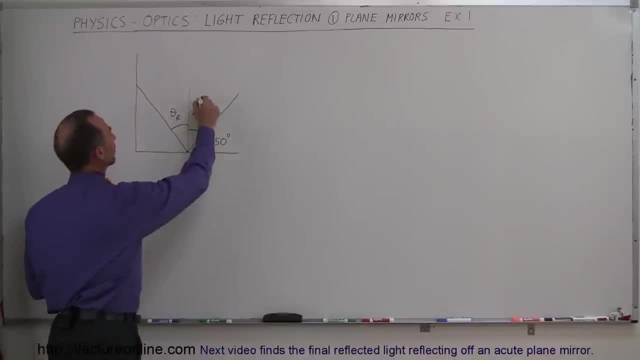 angle has to be 40 degrees. 90 minus 50. that makes this a 40 degree angle, which means that this also must be a 40 degree angle. so what is the angle of incidence against this mirror? right here again, we draw a perpendicular to the mirror and we're trying to find out what this angle is equal to. 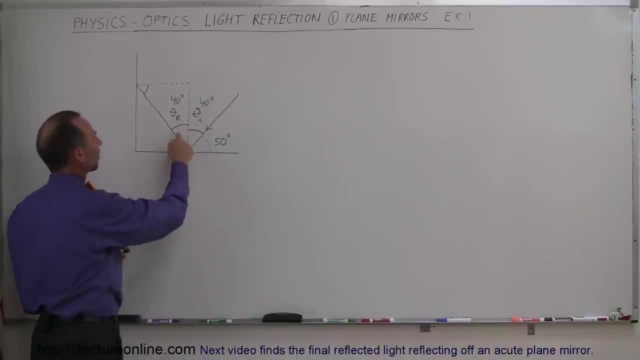 angle of incidence. the best way to do that is to go ahead and say: well, what is this angle right here? this is a 90 degree angle. 90 minus 40 makes this a 50 degree angle. we know that this is the right angle, or 90 degrees, and we know that the sums of the angles of the triangle add up to 180. 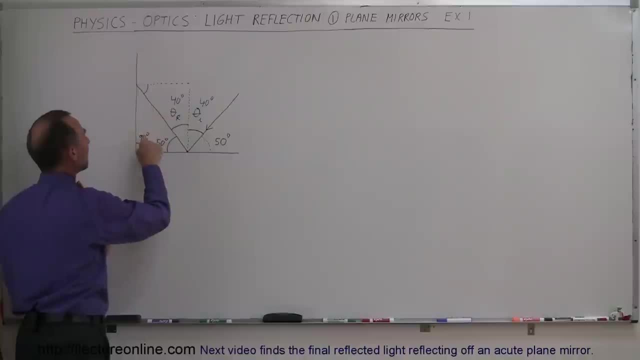 which means that this angle here has to be 180 minus 90 minus 50, so 180 minus 90 minus 50 degrees, which is 40 degrees, which makes this angle a 40 degree angle, which makes this angle, therefore, a 50 degree angle, because the two add up to 90, so this is a 50 degree angle. 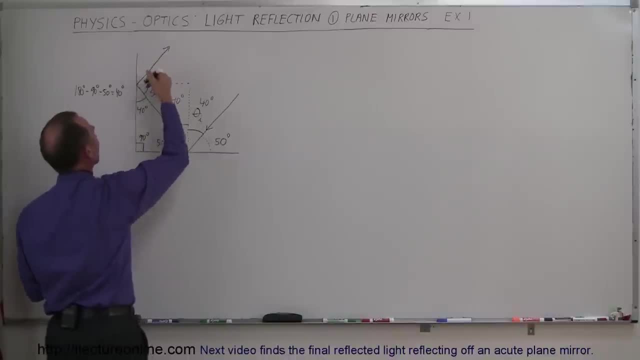 which means that the reflected beam right here will have an angle of reflection over here of 50 degrees, which means that the exiting angle has an angle of 50 degrees above the horizontal. and that's how we follow those. the light rays through a corner reflector, as we call it. that's kind of 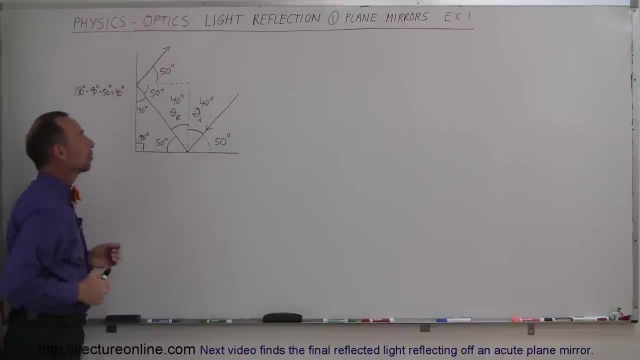 a typical corner reflector where ray comes in and reflects off and then goes back roughly the same direction that it came in on. now we can see how we go ahead and do that in a very simplistic situation. now what do we do if the second mirror is not directly upward or perpendicular to the 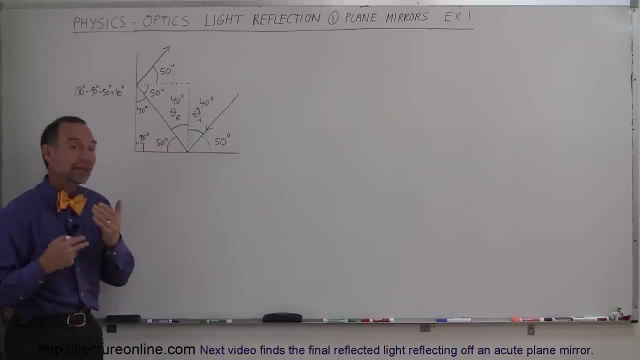 first mirror. what if it's angled inward or angled outward? well then, we have to take care of that differential in the angle, and on the next videos I will show you how to do that.